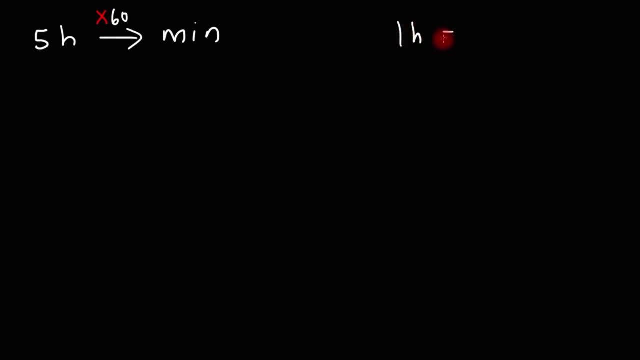 multiply by 60.. The reason being is: one hour is equal to 60 minutes. So here's how you can set up the conversion. In the next fraction, you want to write 60 minutes over one hour. You want to set up the second fraction in such a way that the unit hours cancel, And so it's five times 60 and you. 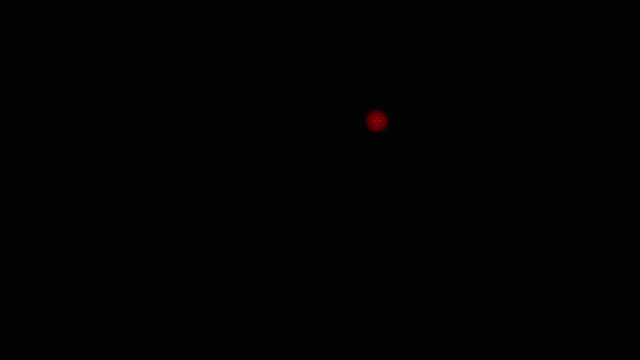 get 300 minutes. So, based on that example, try these two problems: Convert eight hours into minutes And then convert 6.4 hours into minutes. Go ahead and try it. So we have eight hours and there's 60 minutes per hour. So we could cancel those units. 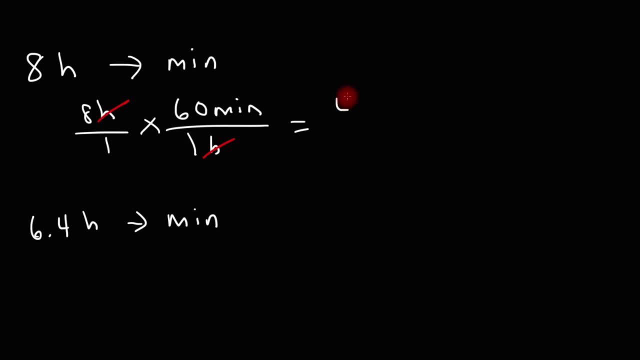 So it's eight times 60.. We know eight times six is 48.. So eight times 60, we just got to add that to the sum of the units. So we're going to convert that to minutes And then convert the zero. That's going to be 480.. So that's the answer for the second example. For the third one, 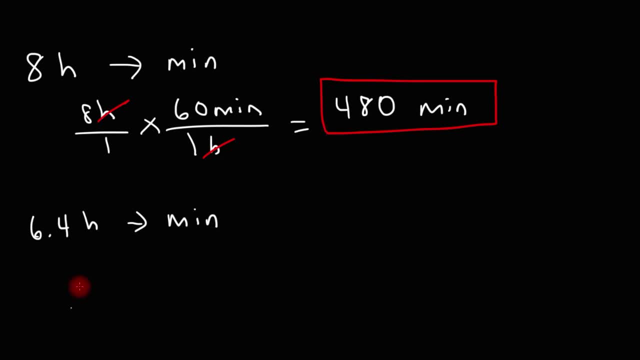 feel free to pause the video and try it yourself. So we have 6.4 hours and we're going to multiply by 60 minutes for each hour. So it's going to be 6.4 times 60. And that's going to give us 384 minutes. 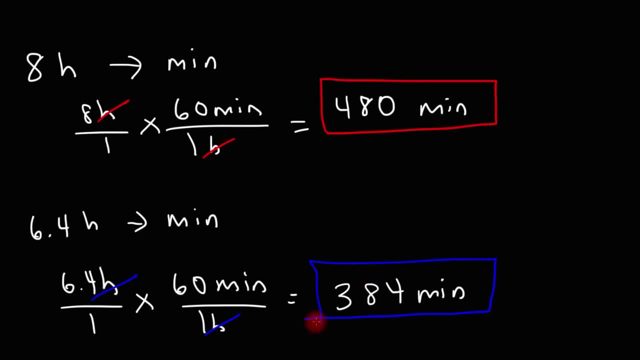 So it's very straightforward to convert hours into minutes, But I'm going to give you a different kind of question now. Now, let's say, if you're given four hours and 20 minutes, how do you convert that into minutes? Feel free to pause the video and think about it for a moment. 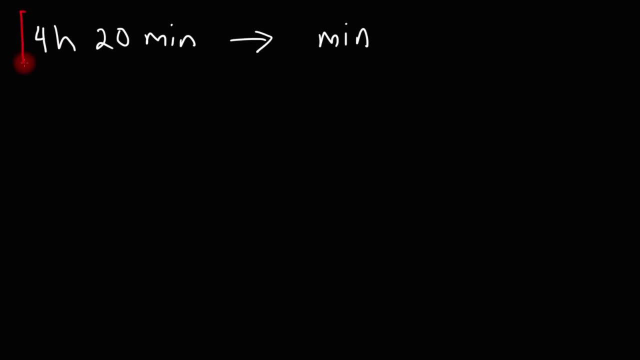 Now what you want to do is convert the hours portion into minutes. So let's do that. So we have four hours And we're going to multiply it by 60 minutes per hour. So it's four times 60.. Four times six is 24.. So adding the zero four times 60 is equal to 240. 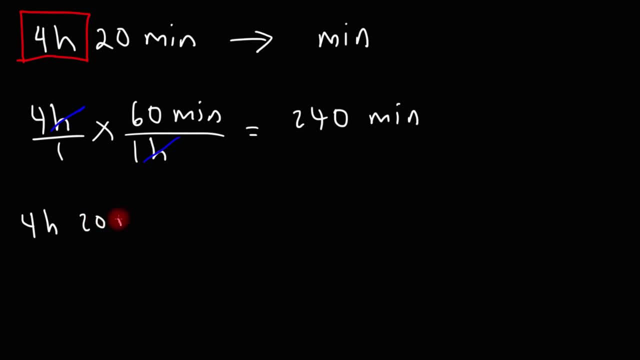 So if we have four hours and 20 minutes, we could replace the four hours portion with the 240 minutes. So this becomes 240 minutes plus the 20 minutes to give us a total of 260 minutes. So that's how we could perform that particular conversion. 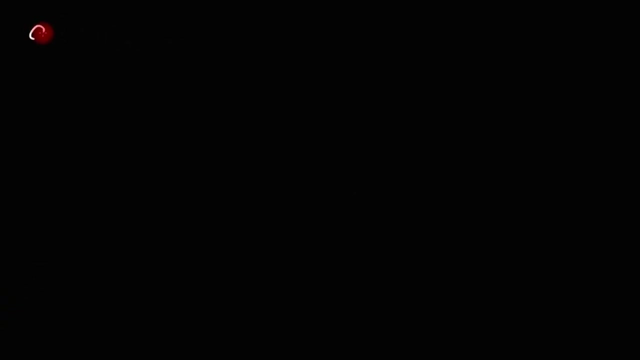 Now let's try another example, Or rather, you could try two examples: Convert nine hours and 30 minutes into minutes, And then convert two hours 45 minutes into minutes. Feel free to pause the video and try that. So let's begin by converting hours into minutes. So we got nine hours. 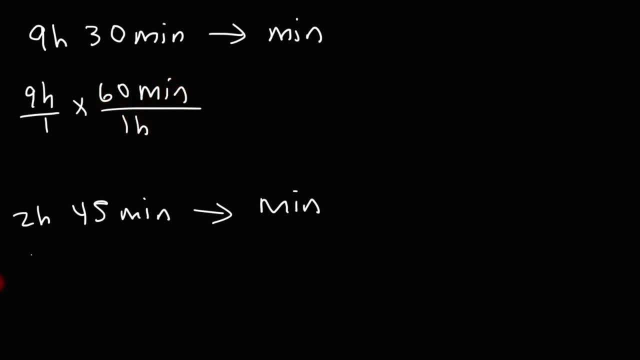 Let's multiply that by 60.. Nine times six is 54.. So nine times 60 is 50. And we've got four hours and 40,. five times six is 540. So nine hours is 540 minutes. So what we need to do is add 540 and the 30.. 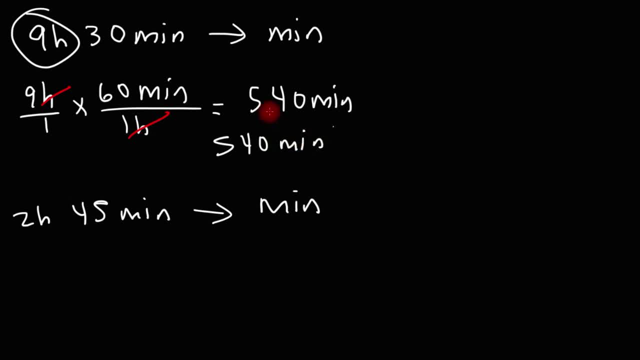 So our final answer is 570 minutes. Now for the next example. let's convert two hours into minutes. What we need to do is add 540 and the 30. So five times 60 is 54. We could also convert two hours into minutes. 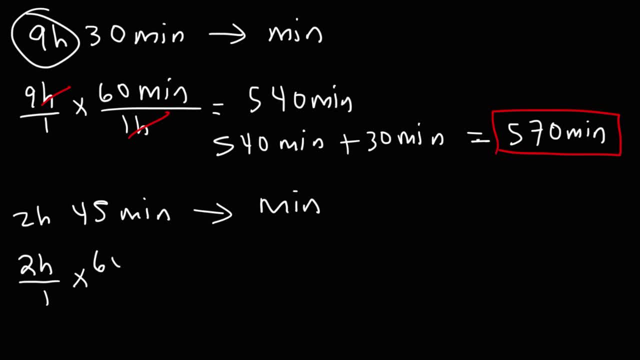 We could also convert two hours into minutes. So five times 60 is 10.. So that's why we're going to do it this way. Let's convert two hours into minutes, minutes. so we just got to multiply by 60. 2 times 6 is 12, so 2 times 60 is going. 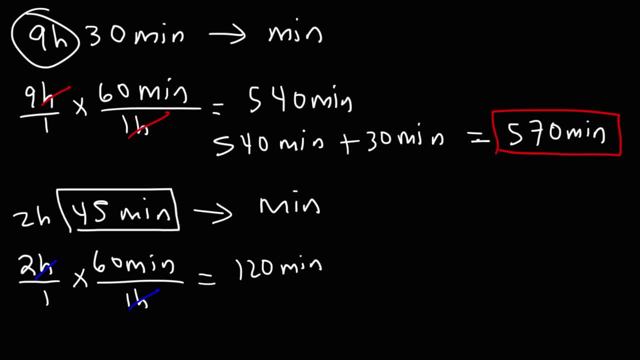 to be 120, and then we need to add this portion. so 120 plus 45, you have 5 plus 0, which is 5, 2 plus 4 is 6. so this gives us a total of 165 minutes. so that's how. 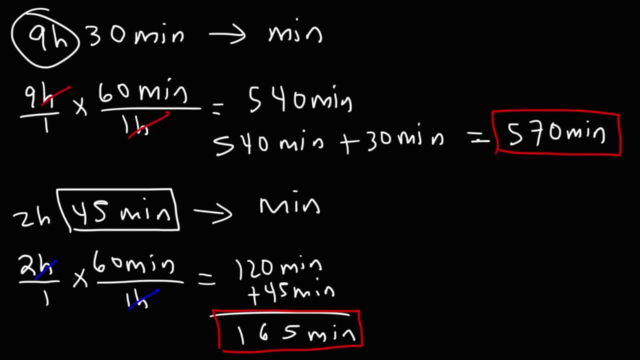 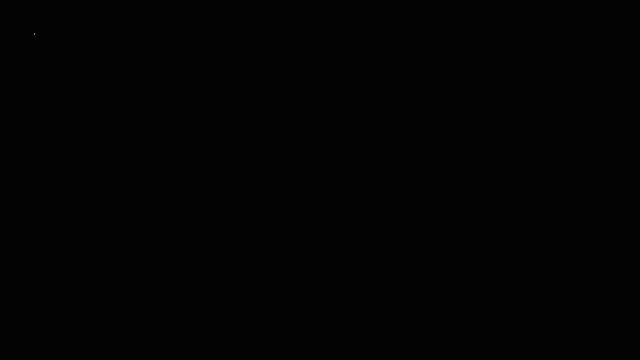 if you have a composite problem with hours and minutes, that's how you can convert it into minutes. now let's talk about working backwards. so let's say: if you're given the time in minutes, how do you convert that into hours? to go from minutes to hours, you need to divide by 60. 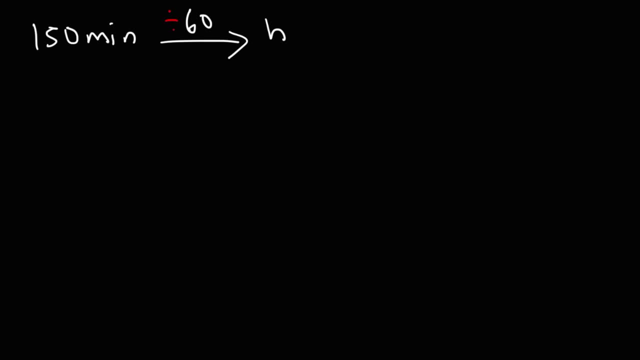 as opposed to multiplying by 60. so here's like a here's something that can help you. if you're going from hours to minutes, multiply by 60. now, if you're going from minutes to hours, just divide by 60. that's a quick and simple way that. 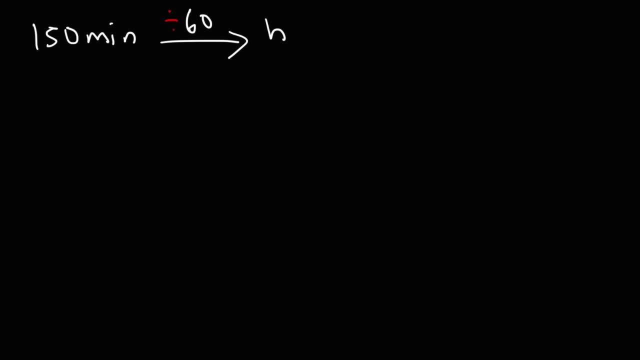 can help you to remember what you need to do in each situation. so let's start with this one, so we have 150 minutes. if you ever forget, the conversion process always helps notice that you have the unit minutes on top, so you need to put the unit minutes on the bottom so that it cancels. so I'm going to put the 60. 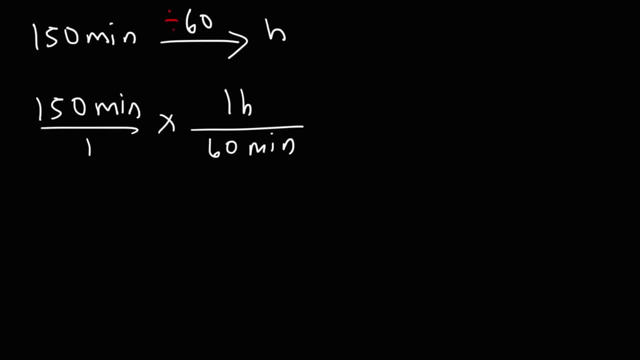 minutes on the bottom, one hour on the top, so that these units cancel, and the fact that the 60s on the bottom it tells me that I need to divide. so 150 divided by 60 is 2.5. so that's the answer for this example. 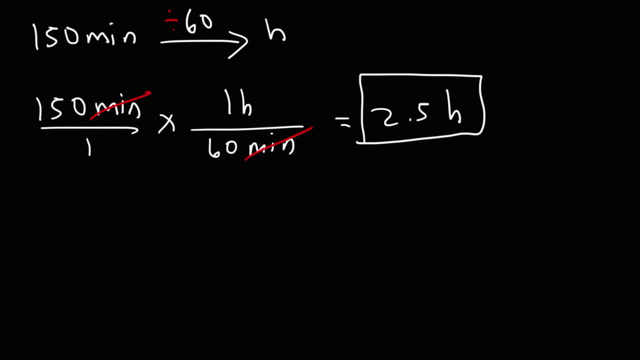 150 minutes is equal to 2.5 hours. now let's try some other examples. convert 280 minutes into hours and also 350 minutes into hours. feel free to pause the video and take a few minutes to work on those two examples. so we're going to. 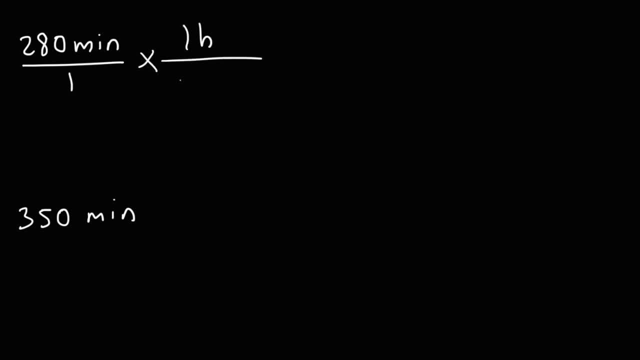 follow the same setup. there's one hour, I mean there's 60 minutes in one hour. so set it up in such a way that the unit minutes cancel. so this is going to be 280 divided by 60 and that is going to be 4.6 repeated, which we can round and say it's about. 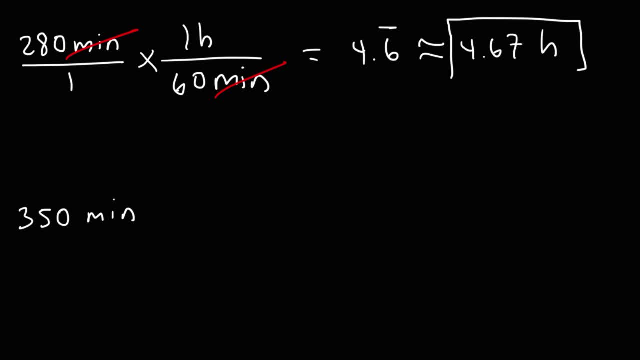 4.67 hours. so that's the answer for the first example. for the next one we're going to follow the same pattern. we're going to multiply by one hour per 60 minutes. so it's going to be 350 divided by 60, and that is 5.83 repeated. so we'll leave. 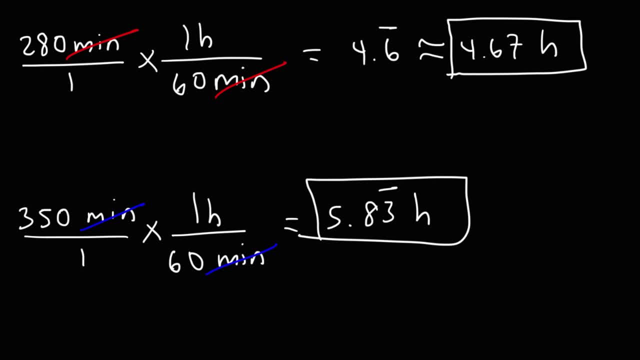 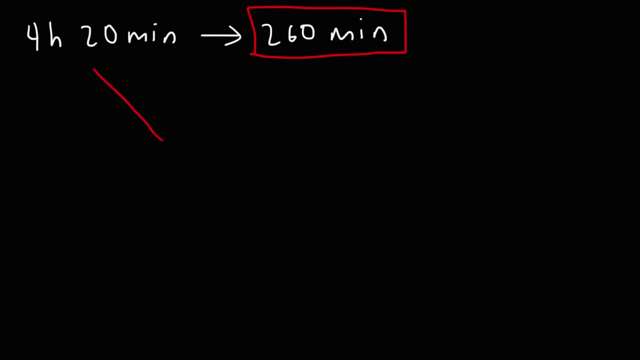 the answer like that. so that's it for those two examples. now here is a question for you. earlier in this video we converted 4 hours and 20 minutes into 260 minutes. now let's say, if you're given the time in minutes, how can you convert it 2 hours and minutes in that form? 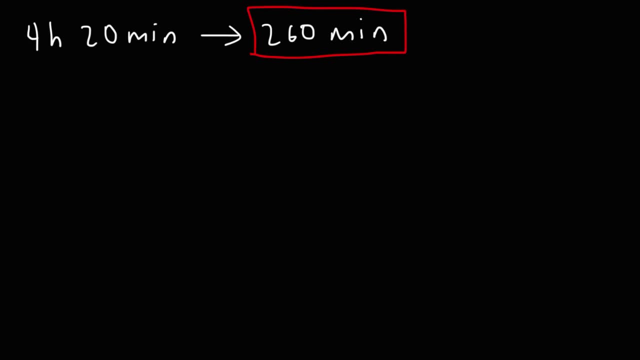 feel free to try this example if you want to go ahead and pause the video and come up with a way to convert 260 minutes back to 4 hours and 20 minutes. so let me tell you what you need to do. first, start with 260 minutes. 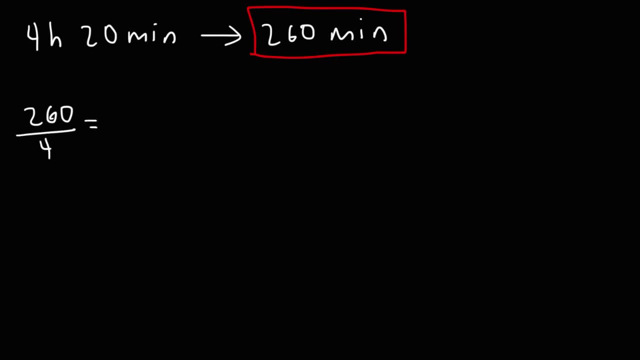 Take your calculator, divide it by 4.. 260 divided by 4 will give you- Actually, I took that back, I did it wrong. You don't want to divide it by 4.. You want to divide it by 60.. 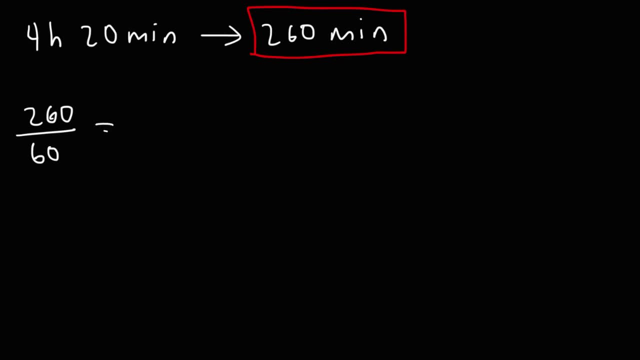 Because you want to convert minutes into hours. So take 260, divide it by 60. This will give you 4.3 repeated, So let's say that's 4.333.. We're going to take away the 4 and save it for later. 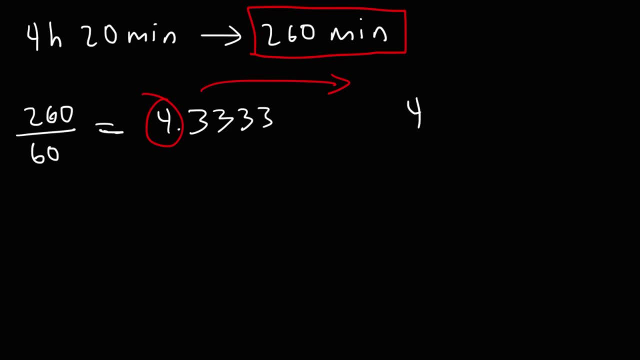 That 4 represents the hours portion of our answer. Now what's left over? The .3333.. Take that value and multiply it by 60. This will give you 19.998 minutes. But keep in mind the 3 should keep repeating. 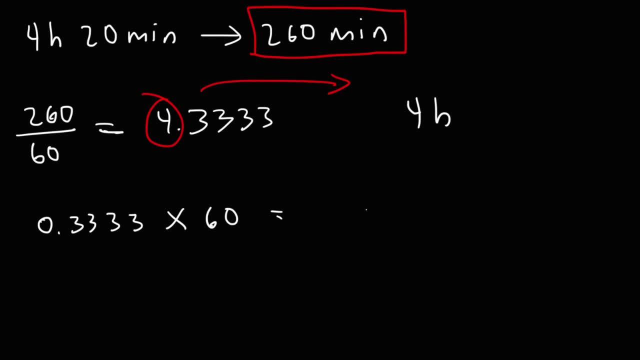 So, therefore, when the 3 goes on forever, It will give you 20.. And so you put this together: 4 hours and 20 minutes. So that's how you can get this answer from this value. That's the process by which you can get that result. 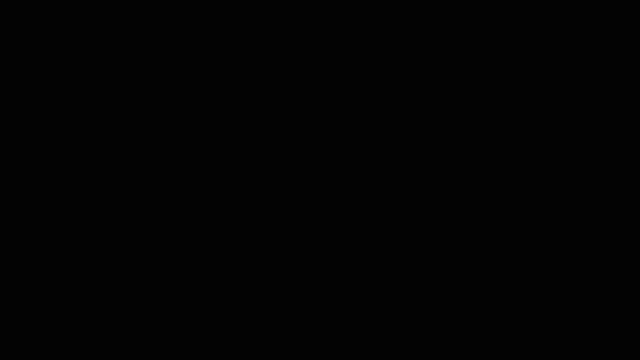 Now, for the sake of practice, let's work on two more examples. Go ahead and convert 325 minutes into Hours and minutes, And then try this one too: 475 minutes. Go ahead and do the same thing. So let's start with 325..